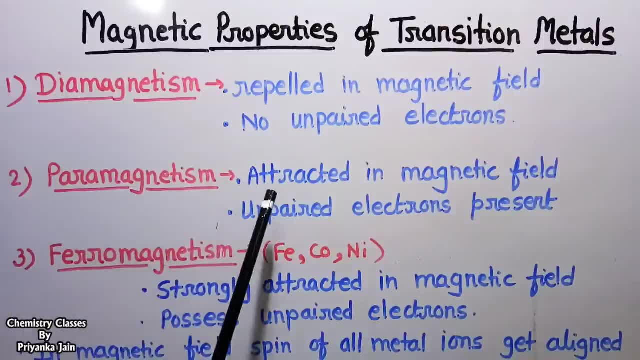 The another is paramagnetism, When a compound is attracted in the magnetic field or it gets attracted towards the magnet. Such a phenomenon is found when the compound possesses Unpaired electrons and due to the presence of unpaired electrons, the compound is attracted in the magnetic field and it is called a paramagnetic compound. 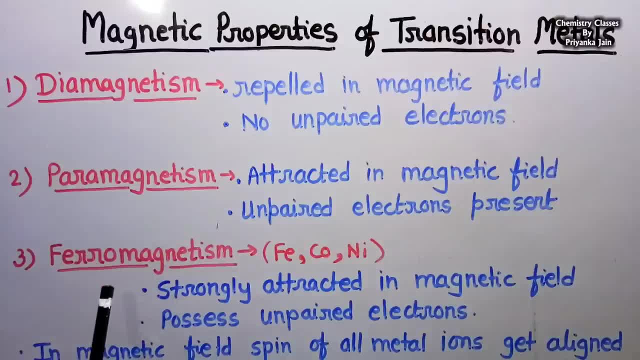 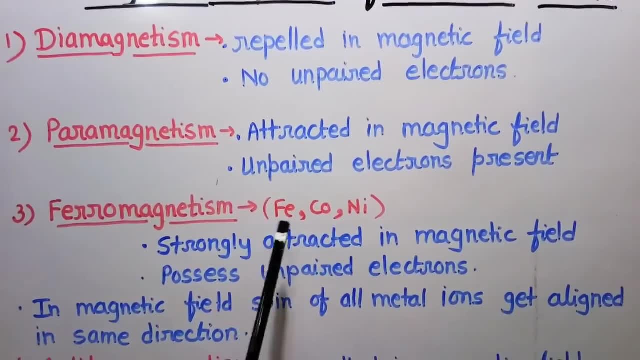 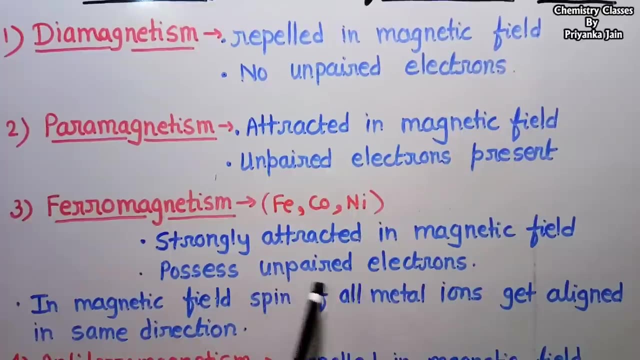 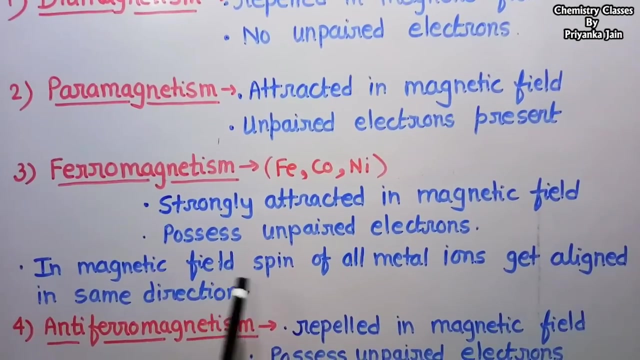 The third phenomenon is the ferromagnetism. Such type of phenomenon is generally found in the iron, cobalt and nickel. Such compounds are strongly attracted in the magnetic field. They also possess unpaired electrons, But in this case the magnetic field. when the compound is kept in the magnetic field, the spin of all the metal ions get aligned in the same direction. 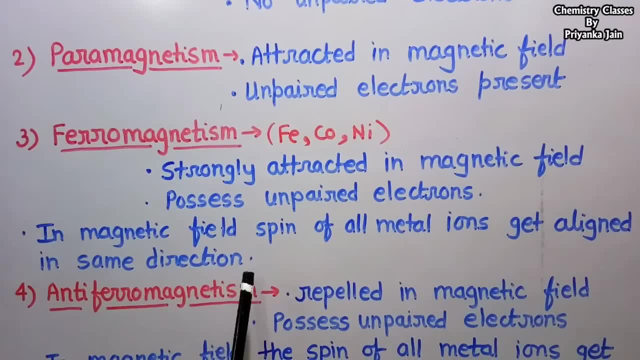 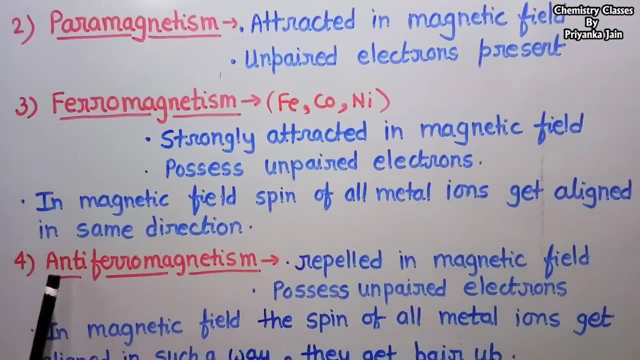 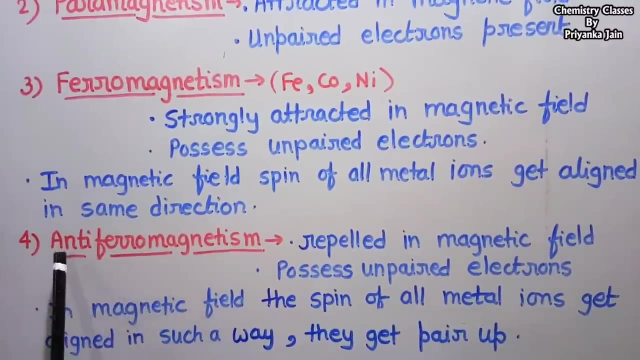 It means the spin of all the electrons get in the same direction, So the compound is strongly attracted in the magnetic field. The fourth phenomenon is the antiferromagnetism. What is this? As from the name anti, It means it is strongly repelled in the magnetic field. 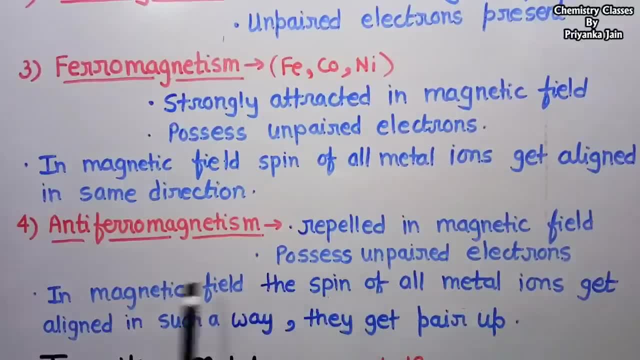 It also possess unpaired electrons. But in the magnetic field The spin of all the metal ions get aligned in such a way that they get paired up. It means all the spin becomes paired, and so the compound is repelled in the magnetic field. 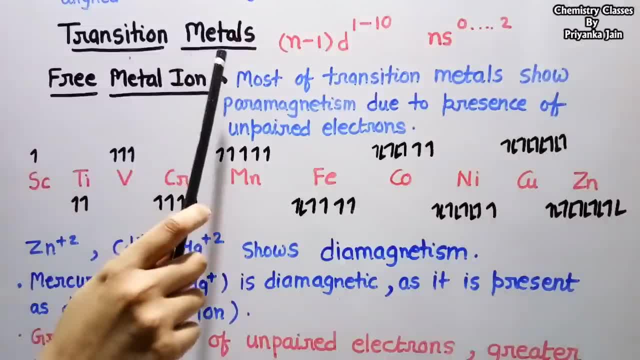 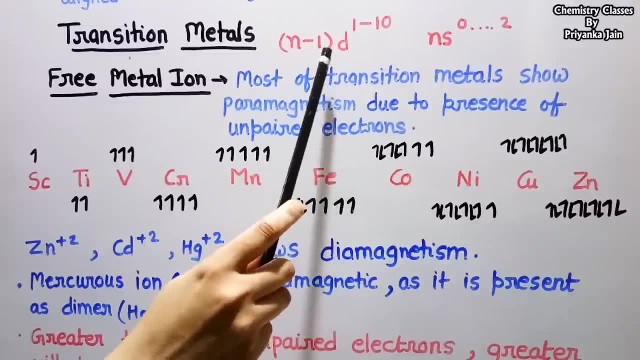 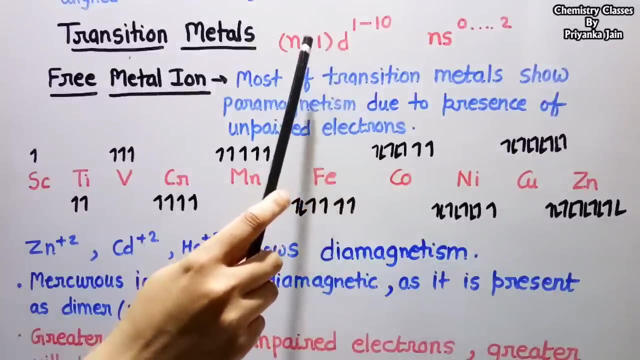 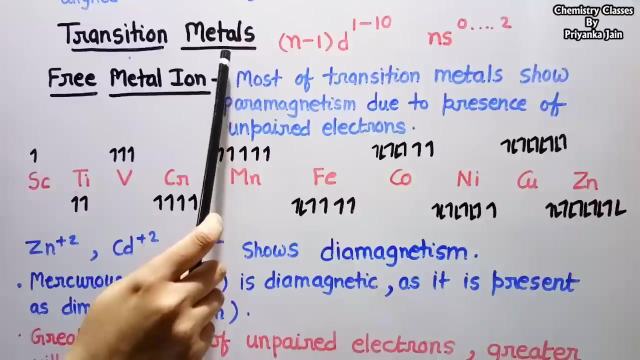 Now we comes to the magnetic property of the transition metals. This is the electronic configuration of transition metals. As we know, in transition metals the electrons are filled in the penultimate d-orbital and these are the electrons that decide the magnetic property of the transition metals. and it is also should be noted that in the case of transition metals, the magnetic property greatly differs when it is in the free state or in the elemental state, or when it gets complexed with the ligands. 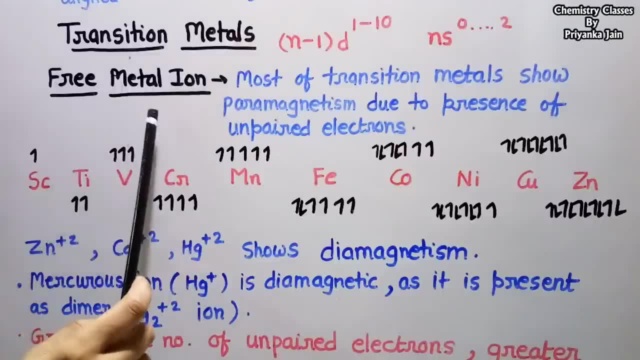 Firstly, we see the magnetic property of the transition metals. We see the magnetic property of the free metal ion. It means when the metal is in the free state, it has not been complexed or it is in the elemental form, Then most of the transition metal shows paramagnetism and this is due to the presence of unpaired electrons, because the electrons are being filled at each level. 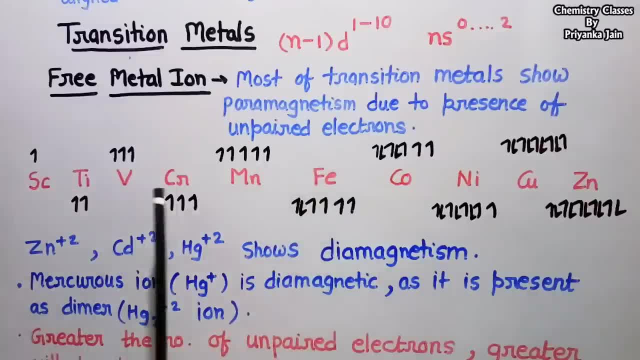 These are filling in the d-orbital. This is the first transition series. These all are the elements of first transition series. Here we have a single electron. Then in the titanium there are 2 electrons and 2 unpaired electrons. 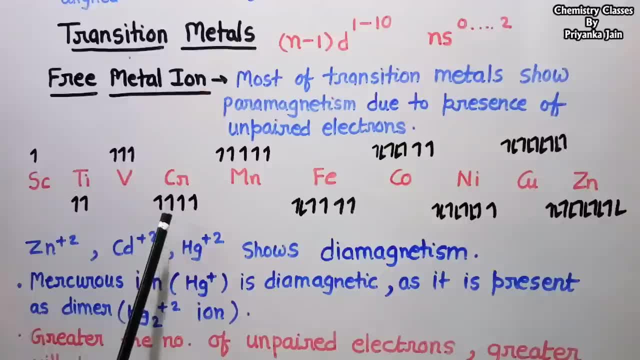 In vanadium 3 and in chromium 4.. The magnet schwierig neuron is composed of an? 4 unpaired electron And in manganese, 5 unpaired electrons are present. This shows the highest paramagnetism of the pre Ten cuanto all. 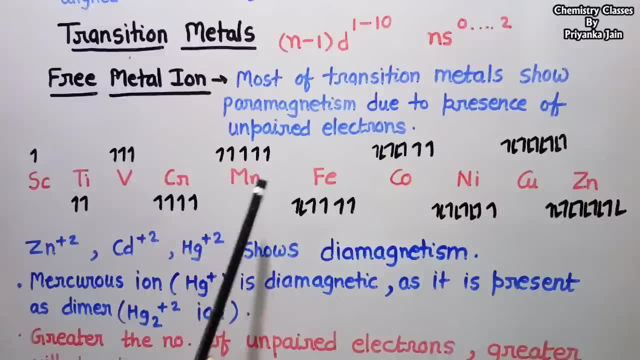 These are the highest unpaired electrons. Then in the iron there are 4 unpaired electrons, 3 in the lithium, frustrated atom and интересно, comatose. The highest paramagnetism of the pre Ten qua all represents the ultra high amongst the신 high proof of Lima. so nс. 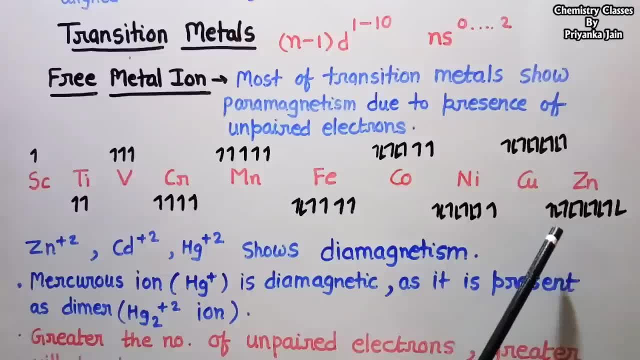 In lady telephone there are right or tidak electron. but in the case of zinc all the electrons are paired up. so zinc does not show paramagnetism, it is a diamagnetic compound. so the magnetic property depends upon the number of unpaired electrons and we can say: in the zinc in 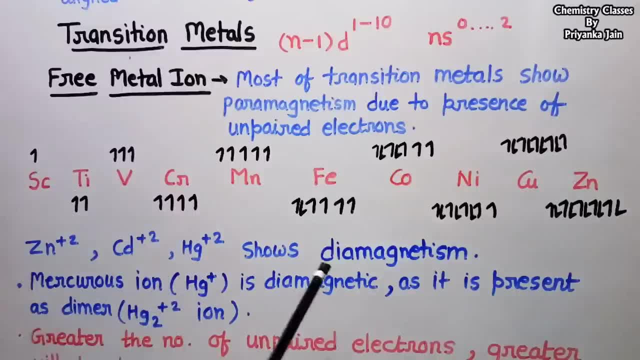 cadmium and in the mercury. they all shows diamagnetism. their plus two ion shows diamagnetism because all the electrons are paired here. one thing should be noted: that in the case of Mercurian it means in HG plus it is diamagnetic. it should be that a magnetic, but it is diamagnetic because in 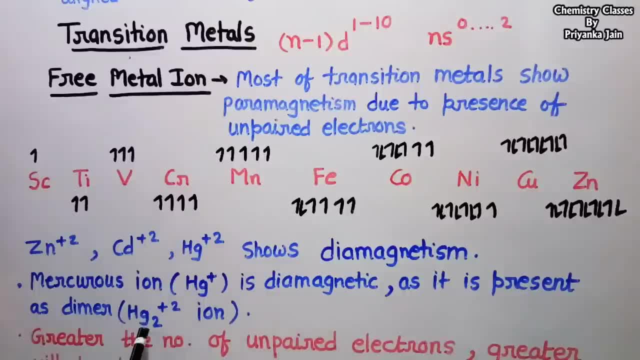 present has a dimer. it means there are two ions, so the spin of both get paired up and it is present as dimer, so it is diamagnetic. the number of unpaired electrons, greater will be the paramagnetism minutes less going to run better than definite because of the heat takes two to the 했는데. the resistance. 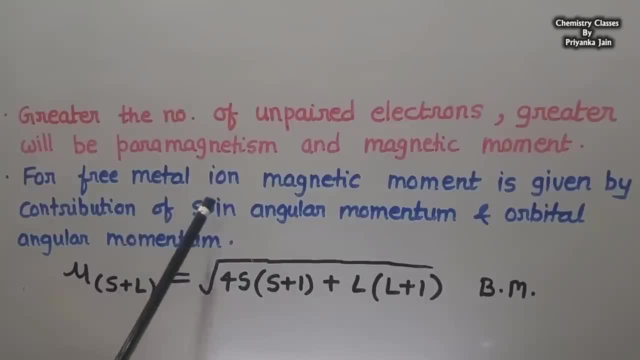 will be the magnetic movement. For the free metal ion the magnetic movement is given by the contribution of spin angular momentum and the orbital angular momentum because there is spin orbital coupling. So the total magnetic movement is given by the under root 4s s plus 1. 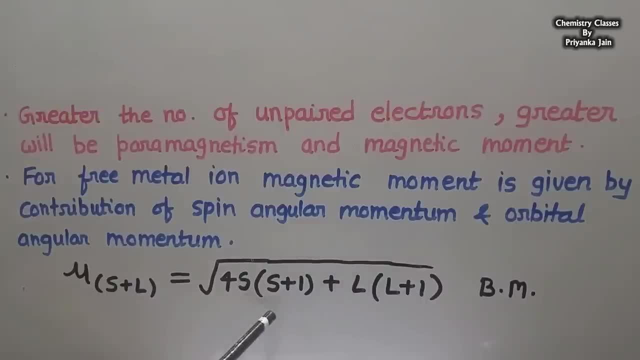 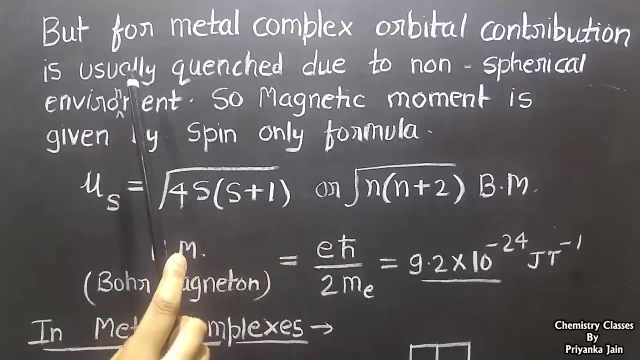 plus l, l plus 1, where s is the spin quantum number and l is the angular quantum number or orbital quantum number and bm is the pore magneton Metal. complex: it means when the metal get complexed the orbital contribution to the magnetic movement is usually quenched. it means 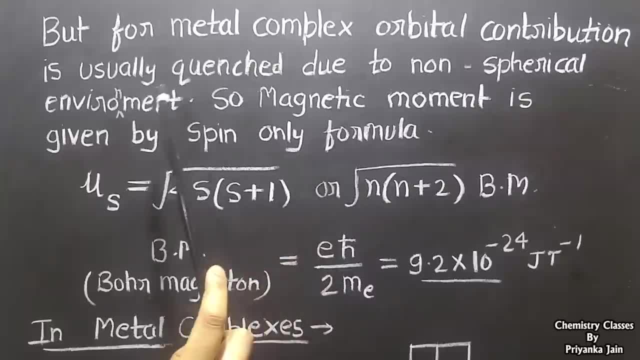 it becomes equal to 0.. Why? Due to the non-spherical environment. About this quenching of the orbital contribution we will study later. Firstly, we see that in such cases the magnetic movement is given by the under root 4s s plus 1 plus l l plus 1 plus l l plus 1 plus l l plus 1. 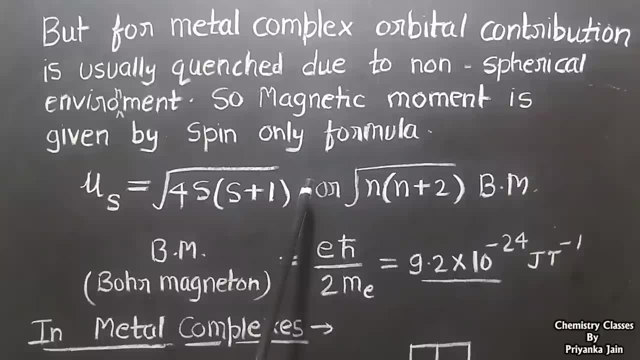 is usually given by the spin only formula. What is this formula? That is, mu s is equal to under root 4s s plus 1, or it may be under root n, n plus 2 bm, where n is the number of unpaired electrons. 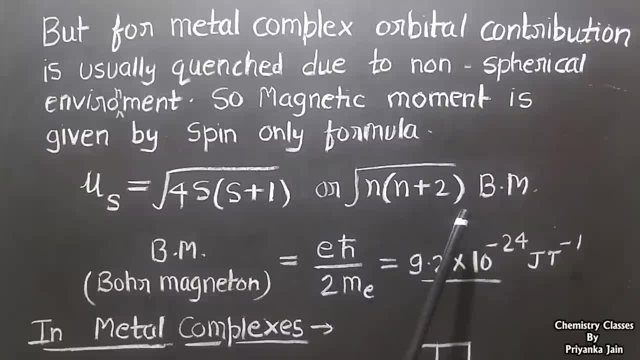 s is the spin quantum number and bm is the pore magneton, that is, the unit of the magnetic movement. The pore magneton is given by the formula e, h bar upon 2me, Where h bar is equal to h upon 2 pi. e is the charge of the electron and me is the mass of the. 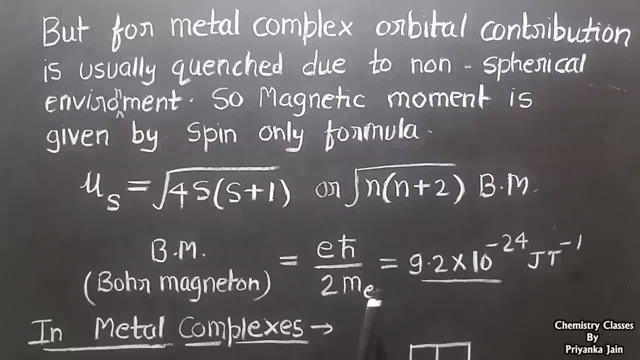 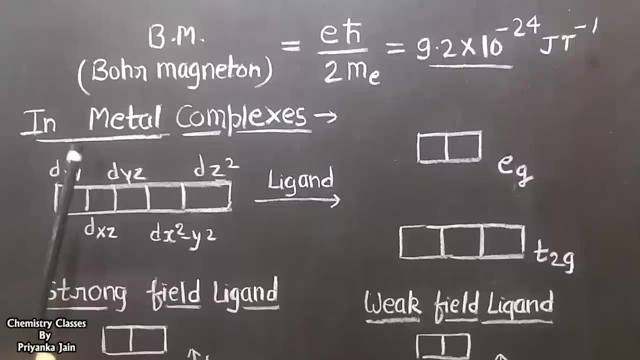 electron, and all of these are constant. So its value is equal to 9.2 into 10, raised to the power, minus 24 joule per tesla. Now, one thing should be noted. why this? is the change in the behavior of the transition metals when they get complexed with the 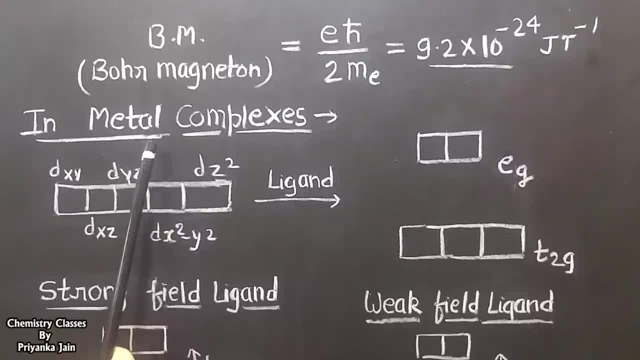 ligands, and this can be explained on the basis of the crystal field theory. What is crystal field theory? According to the crystal field theory, when the metal is in the free ion, when it is in the free state, it has not combined with the ligand. All the 5d orbitals. 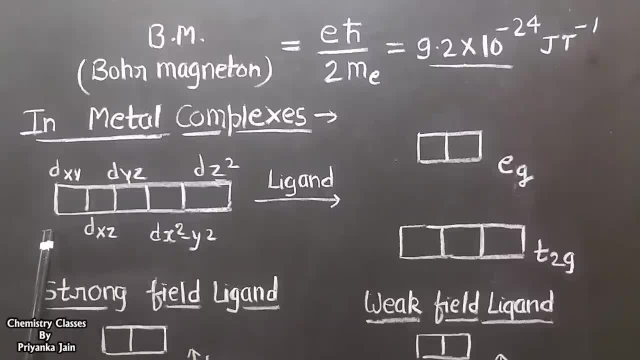 are degenerate. It means all have the same energy, So the electron get a path for the rotation around the nucleus and it forms a solid. wiem How to solve this. Just look at the diagram for the solution and it will be easier to. 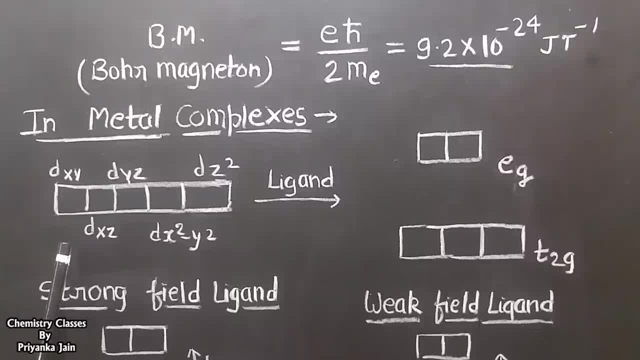 the orbital angular momentum and hence the magnetic movement is resultant of the spin and the orbital angular momentum. But when the ligand is complexed with this metal, it means when the ligand comes near the degeneracy, of these five orbitals is removed. it means 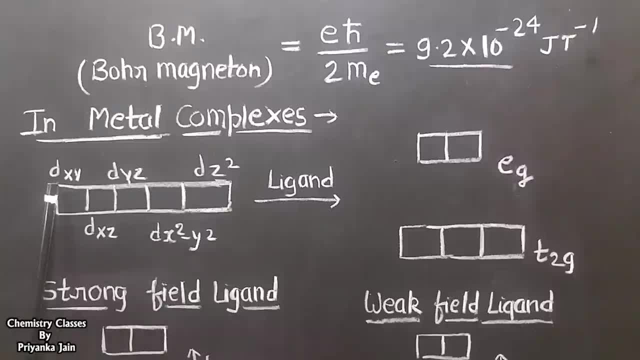 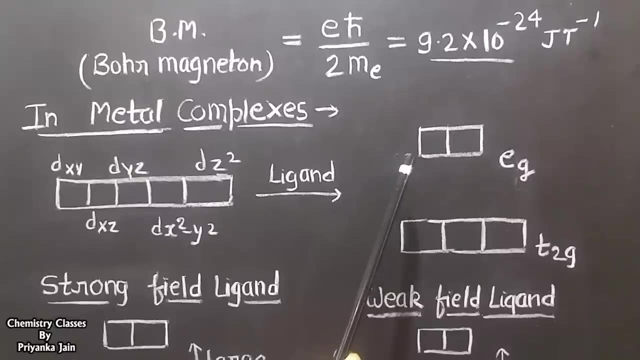 the three of these d orbitals that are dx, dy and dz that get lowered in energy, and these three are degenerate, So they are called t2g orbitals, while two another that are dx square and dz square get higher in energy and this forms the eg set of the orbitals. 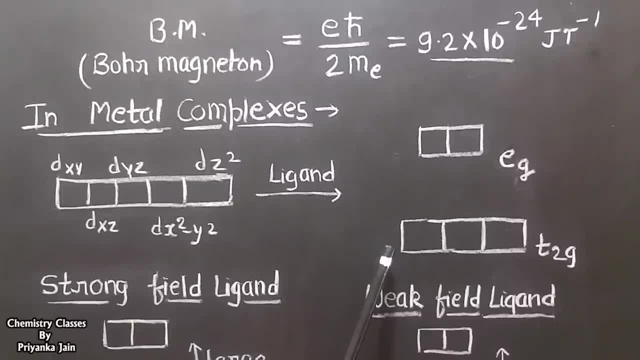 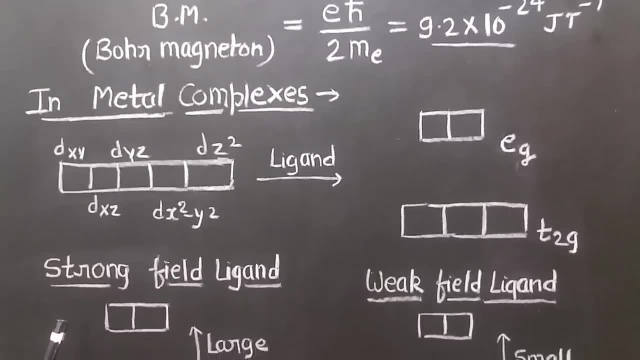 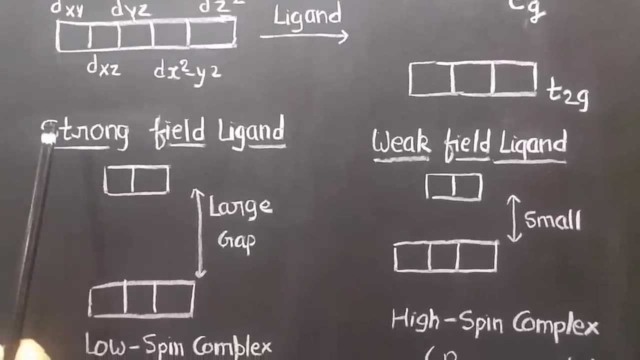 So we get two different sets that are t3g and t2g, 2g and eg, and there is a difference of energy between these two levels. now two things can be happen. when the ligand is strong field, it means it is high field ligand, similar to cyanide or co. 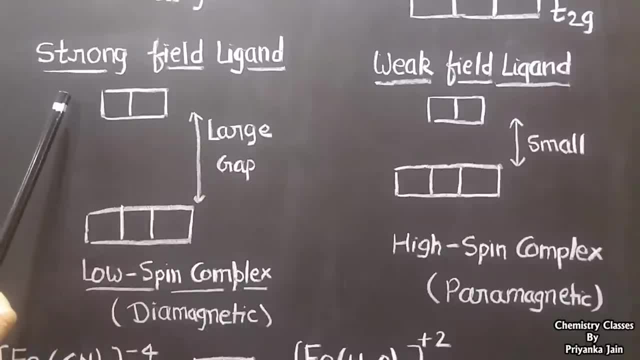 carbonyl. these are strong field ligand and these can cause the high splitting of these d orbitals. it means the energy gap between these two levels is very much higher when such elegant is complex to the metal. so the energy of t2g level is very much low, while that of easy level is very much. 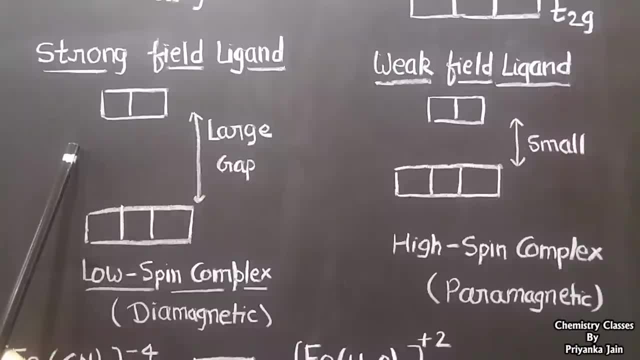 high in the case of octahedral complex. we are taking here octahedral complex in the consideration, so the energy required to jump the electron in this level is very much higher as compared to energy that is needed for pairing the electrons in these levels. so the electron wants to pair up. 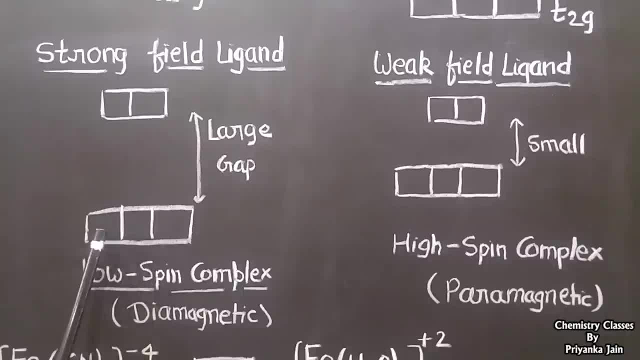 it means they firstly get fill in this t2g level and then they pair up and then they comes to the easy level. so the complex that we get is of low spin type. it means the maximum electrons get paired and we get a low spin complex, and such complexes are mostly diamagnetic. now we 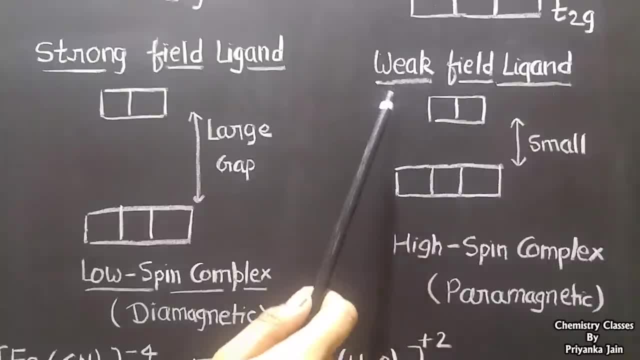 the case of weak field ligand. when the ligand is weak field, such as chloride ligand or oxide ligand. in such cases the splitting is very small. the energy gap between these two level is very small, so the electrons can easily jump to this easy level. and the electrons firstly. 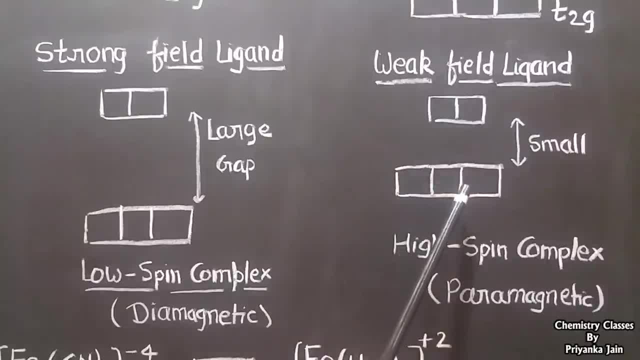 go to t2g level, then go to e, g and then they pair up. so we get a high spin complex. it means maximum number of electrons remains unpaired and we get a paramagnetic complex. so this decides that whether a compound will be low spin or high spin, 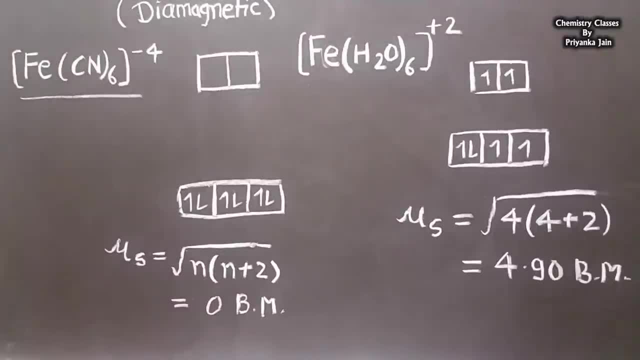 we can see it with the help of an example. if we take the iron and we take its two complex, one is this type of complex, that is, fe, cn6 minus four charge. this is a complex full. Просто It means that the amount of electrons remains unpaired and we get it paramagnetic complex. so this: 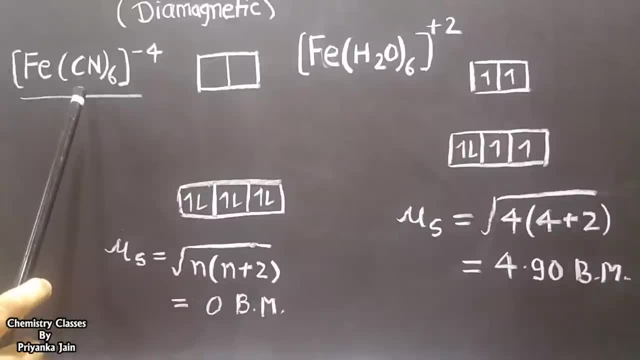 four charge. This is a complex with the strong field ligand because cyanide is a strong field ligand and it causes a large splitting of the two levels. This is a large splitting So the electrons all get paired up in this T2G level because it requires higher energy to jump in the 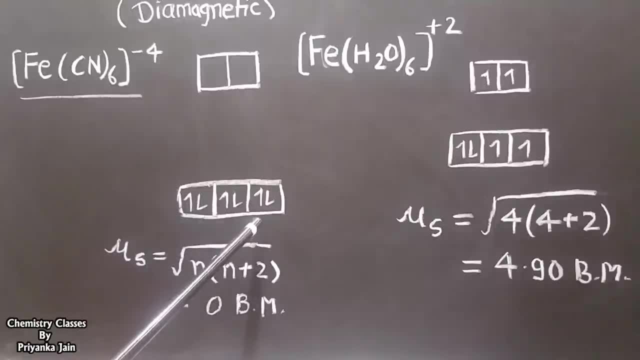 EG level. So all the electrons get paired in the T2G level and the mu s it means the magnetic moment spin only formula. We get under root n, n plus 2 and it becomes equal to 0, because there is no unpaired electrons. So this compound is diamagnetic. and if we see another compound that 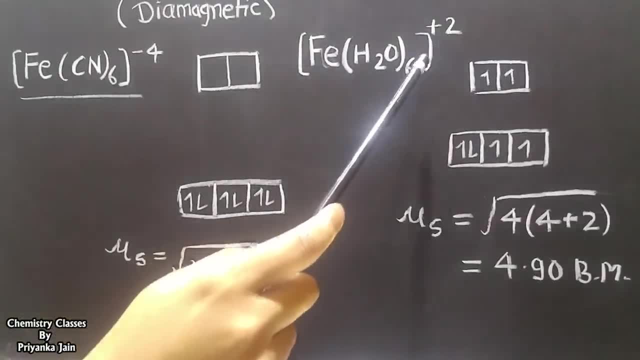 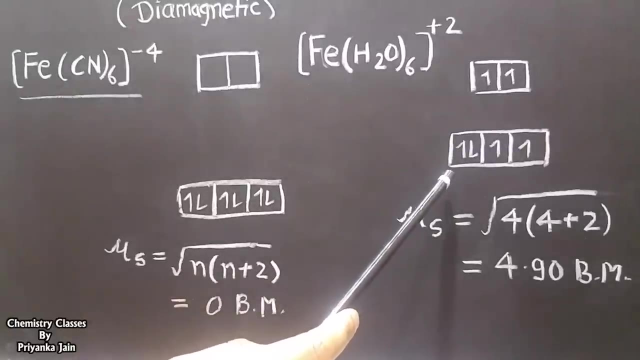 is FeH2O whole 6 plus 2 charge In this compound. water is present as a ligand and this is a weak field ligand So it causes a small splitting, very small splitting of the two levels. So this is a large splitting of these two levels, So the electrons can easily jump into the EG level. Then 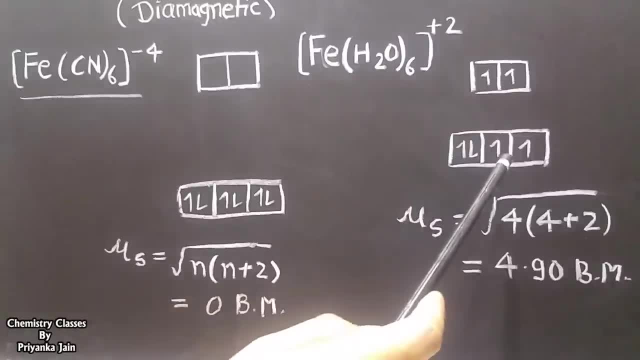 becoming the pair up in this level. So we get this type of structure. It means four unpaired electrons are present here, So the magnetic moment is given by under root 4, 4 plus 2, that is 4.90 Bm, and such a compound is highly paramagnetic. 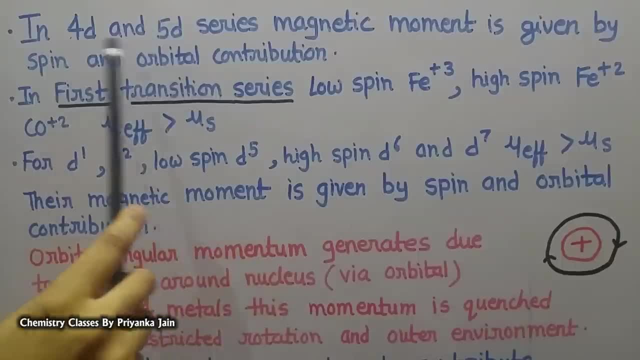 the magnetic movement is given by the spin and the orbital contribution. But in the case of first transition series the magnetic movement is generally given by the spin only formula. But there are some cases like low spin Fe plus 3 ion. high spin Fe plus 2 ion CO plus. 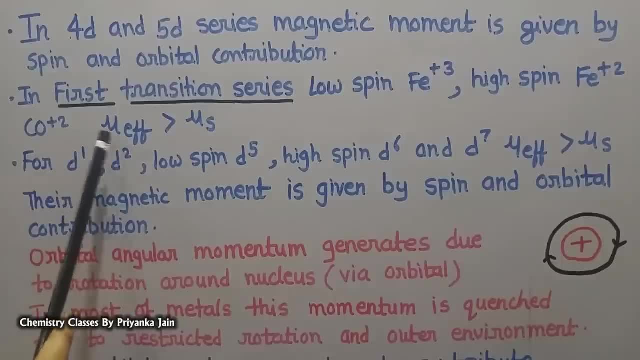 2 ion. In these cases, the mu effective, or the magnetic movement that is observed, is usually greater than the mu? s. If we see the transition series carefully, then we find that for the d1, d2, low spin, d5, high spin, d6 and d7 complexes, mu effective is greater. 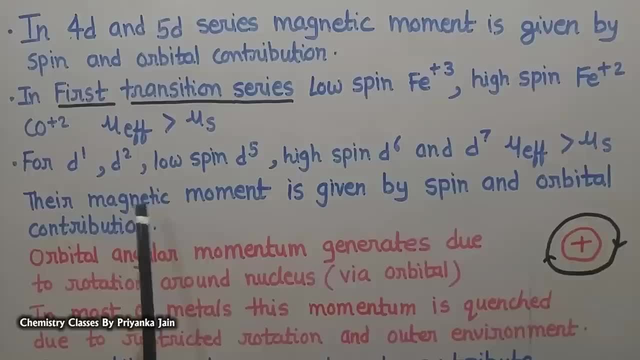 than the mu s. Why? Because in these cases the magnetic movement is given by the combination of both the spin and the orbital angular momentum. So why it happens that in some cases we get the magnetic movement by only spin formula and in some cases we use both the spin and the orbital contribution. The reason for this? 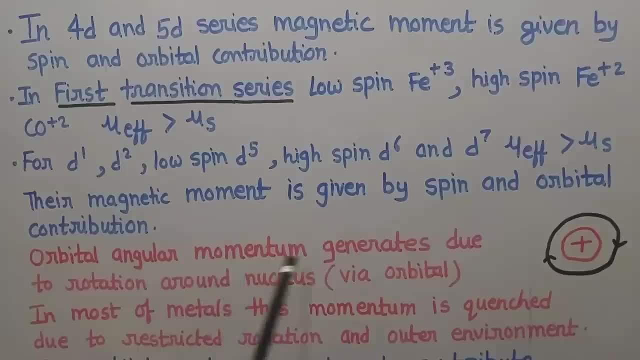 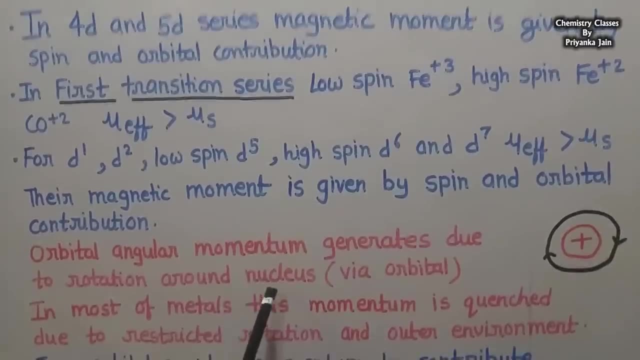 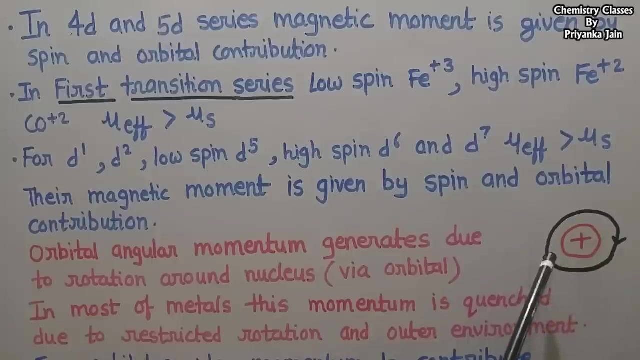 is that the orbital angular momentum generates due to the rotation of the electron around the nucleus and this rotation happens via the orbitals. It means this is a nucleus and the electron rotate around the nucleus And it is present in the orbitals. So it will rotate via the orbitals around the nucleus. 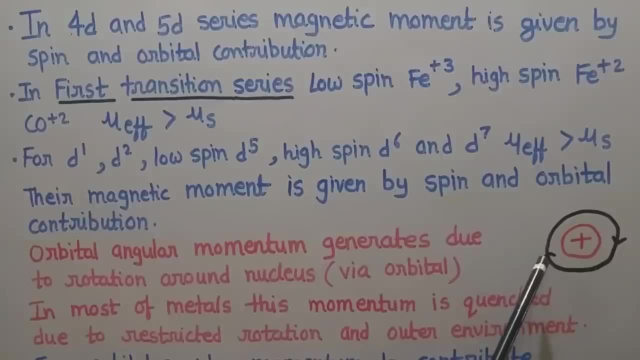 And when it rotates then only the orbital angular momentum generates. If there is no path for the electron to rotate, then it cannot produce the orbital angular momentum. So in most of the metals this angular momentum is usually quenched. Why? Because of the rest. 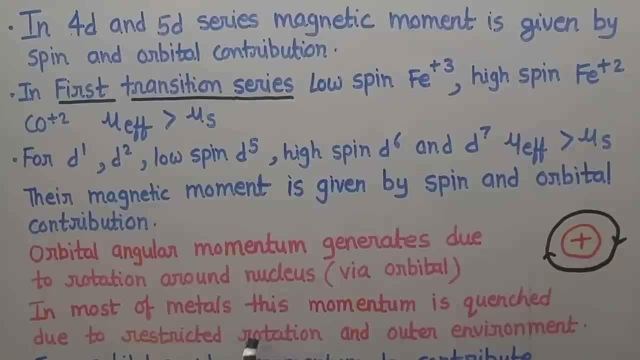 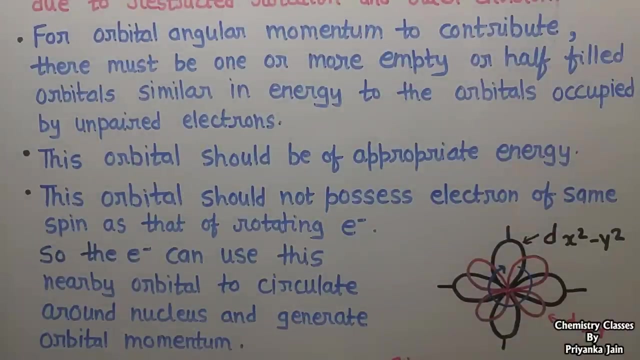 restricted rotation. It means the rotation of electron is restricted because it does not get the path for the rotation. This is somewhat due to the shape of the d orbital and somewhat due to the effect of the ligands or the outer environment. So for the orbital, 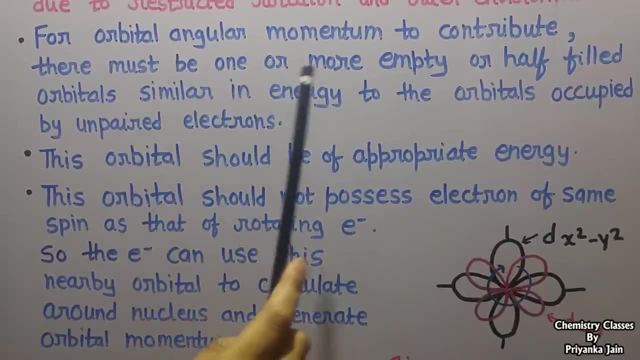 angular momentum to contribute, there must be one or more empty or half filled orbitals similar in energy to that of the orbitals occupied by the orbital angular momentum. Such a orbital should be present for the orbital angular momentum to contribute, And this orbital should be of the appropriate energy. It means its energy should be similar to that of the 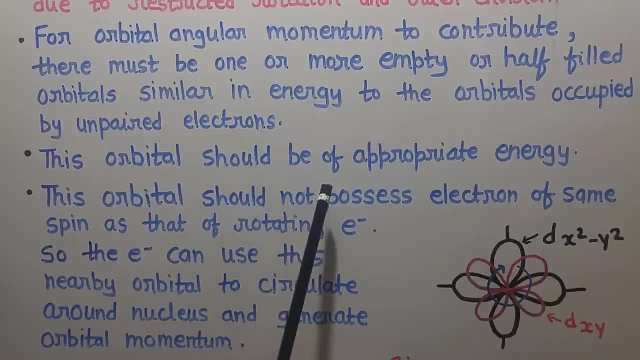 orbital that possesses the electron and of the same symmetry, And this orbital should not possess the electron of the same spin as that of the rotating electron, So that the electron can use the same spin as the rotating electron, So that the electron can 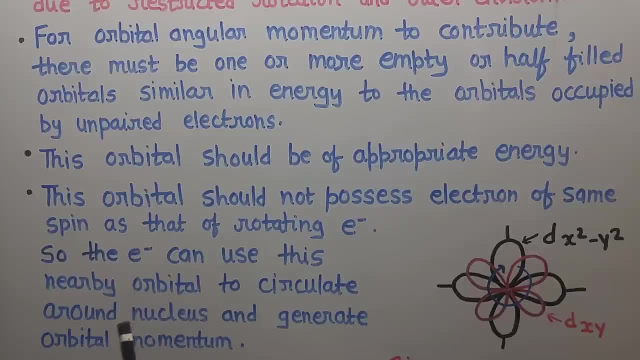 use this nearby orbital to circulate around the nucleus. It means it provides a path for the electron to circulate around the nucleus And in this way it can generate the orbital momentum. For example, if we see these two orbitals, this is dx square minus y square. 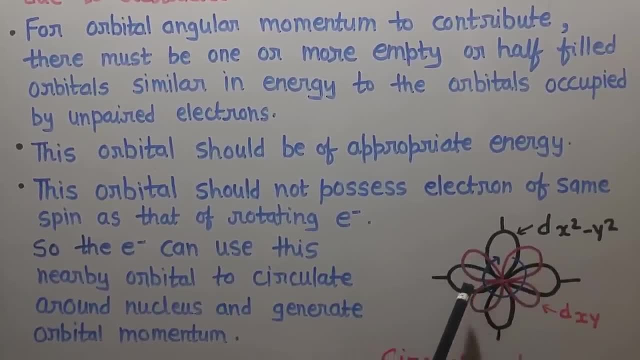 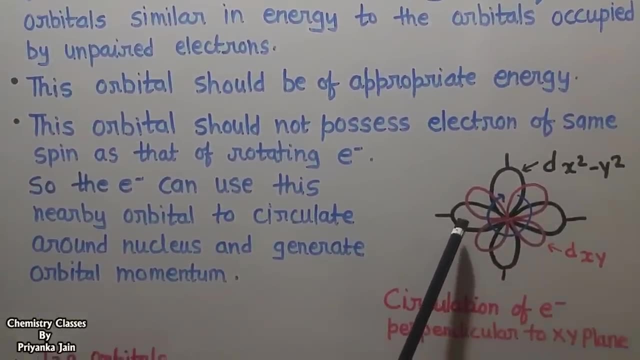 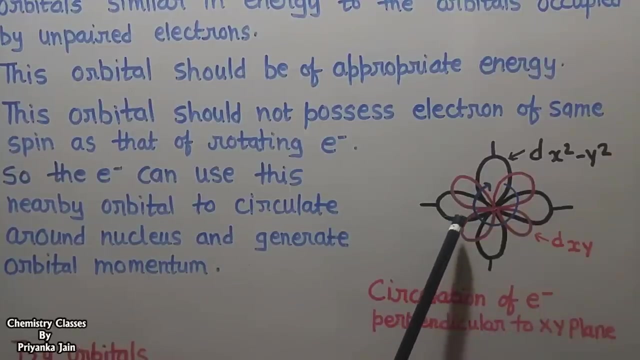 orbital, That is, we have denoted by the black color, and this red colored is dxy orbital. Now, these two orbitals are of almost similar energy and this can be transformed by rotation around 90 degree, So these provide a path to the electron for the circulation. This 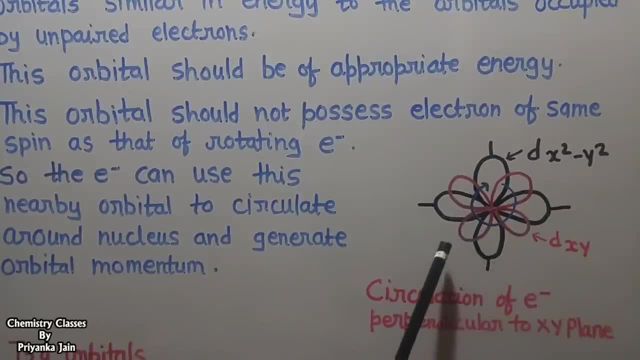 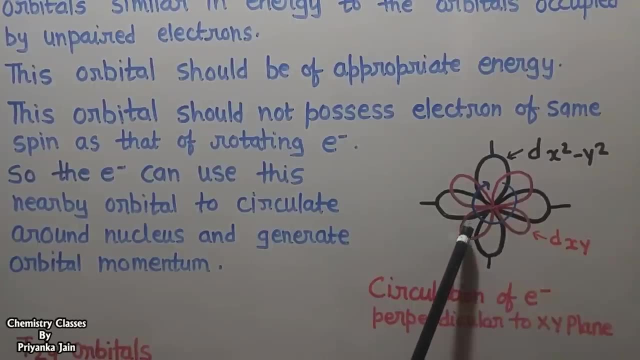 blue colored line shows the circulation of the electron when we apply a field perpendicular to the X Y plane, And this orbital should not possess the electron of the same spin so that this bebty rotation can be performed. This orbital should not possess the electron. 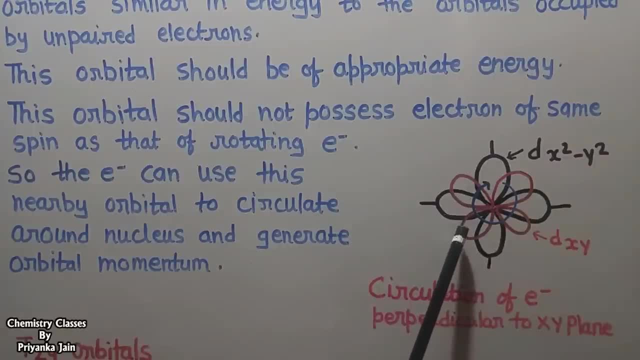 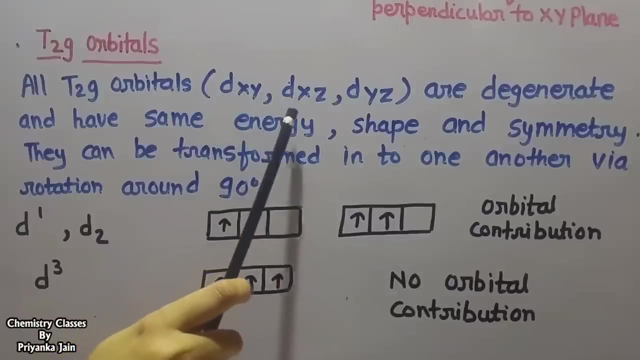 of the same spin Enендingться, sorted as follows: that power small angle control circle. this electron can move by this orbital T2g orbitals. all the T2g orbitals, dxy, dxz and dyz, are degenerate and have the same energy, shape and symmetry and they can be. 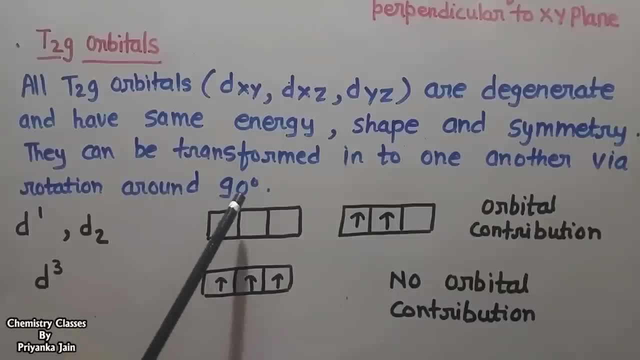 transformed into one another by rotation around 90 degree. So if we see the d1 and d2 configuration, in d1 there is one electron present in T2g level and these two orbitals are vacant. So the electron can use this orbital to rotate around the nucleus and in this case there are two. 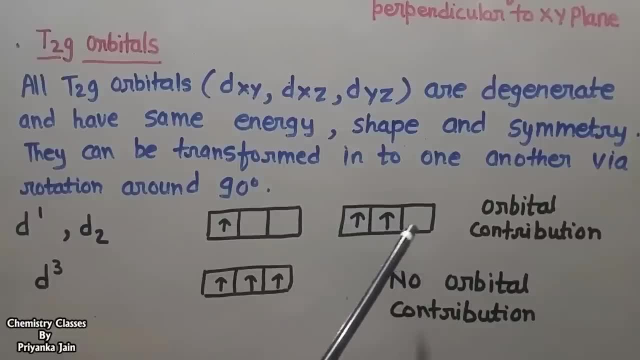 electrons and this orbital is empty, So the electron can rotate via this orbital. So these two makes the contribution, orbital contribution towards the magnetic movement, While in the case of d3 configuration there are three electrons present in T2g level. So these two electrons 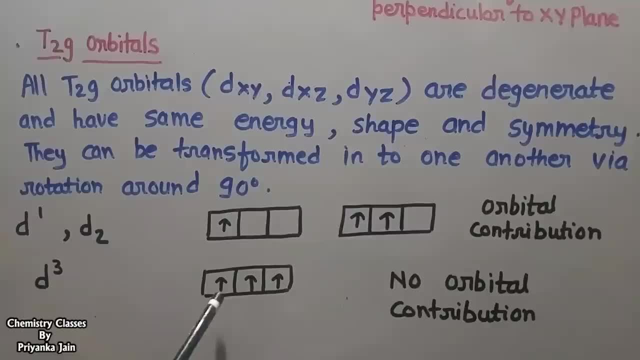 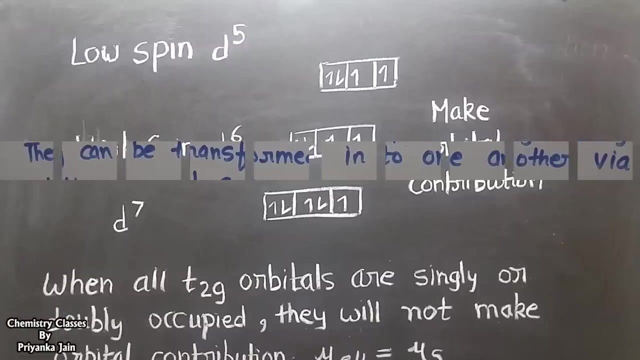 are the three electrons in the three T2g orbitals, So all are of similar spin. So there is no vacant T2g orbital, So there is no path and hence no orbital contribution, And in this case the magnetic movement will be given by only spin formula. Now low spin, d5 configuration. 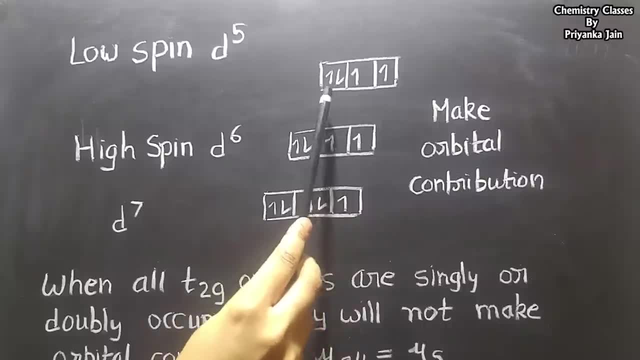 this is the stage of the T2g level. There are four electrons and two electrons in this orbital. It means one electron with the inverted spin in this orbital, While in these two orbitals there is no electron with the inverted spin. So it provides a path for this inverted electron. 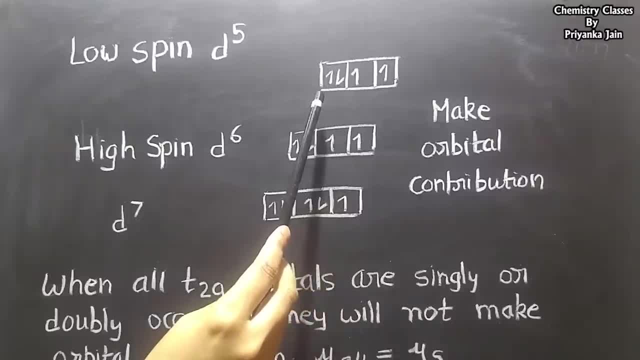 to rotate and this makes a contribution, orbital contribution, towards the magnetic movement. Similarly, in the high spin d6, there is one electron with the inverted spin in this orbital, while these two do not have. So it provides a path for this inverted electron to rotate. So 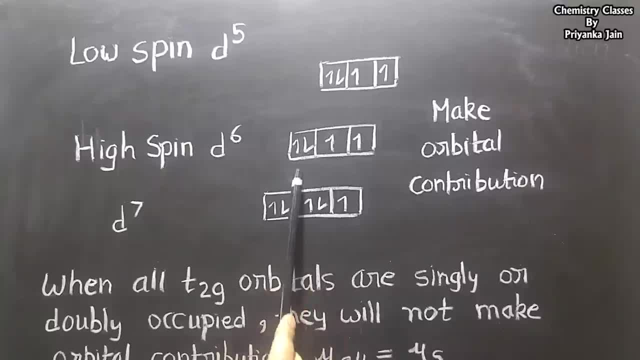 it provides a path for this electron to rotate. Similarly, in d7 configuration these two have two 2 electrons. It means this one with the inverted spins and these two do not have. So it provides a path for this electron, or this electron, to rotate around the nucleus. 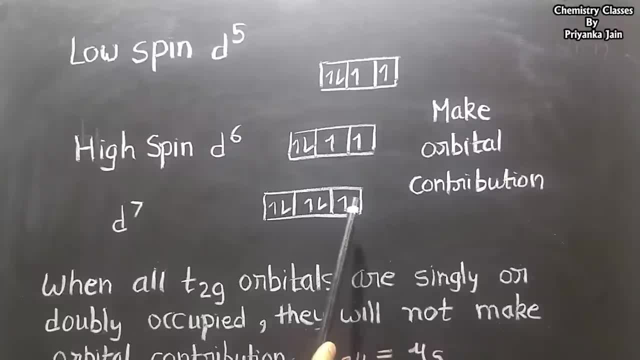 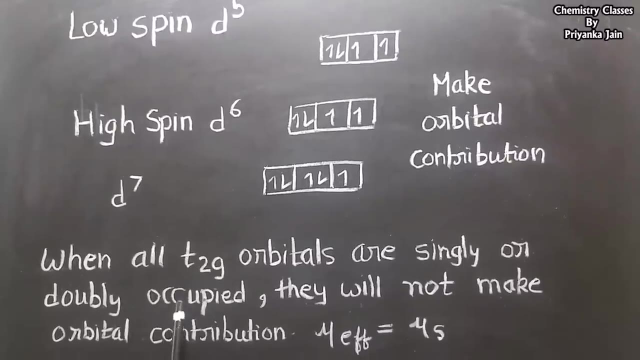 So all of them will make the orbital contribution towards magnetic movement and will have the magnetic movement higher than the spin only formula. But when all the T2G orbitals are singly or doubly occupied it means there are 1,, 1 electron. 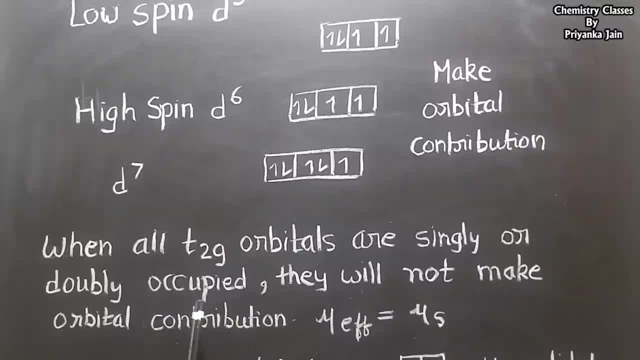 in all T2G orbitals or 2, 2 electrons in all T2G orbitals, then there is no path for the rotation of the electron, So they will not make the orbital contribution toward the magnetic movement. So the mu effective will be equal to mu s. It is also affected by the geometry. 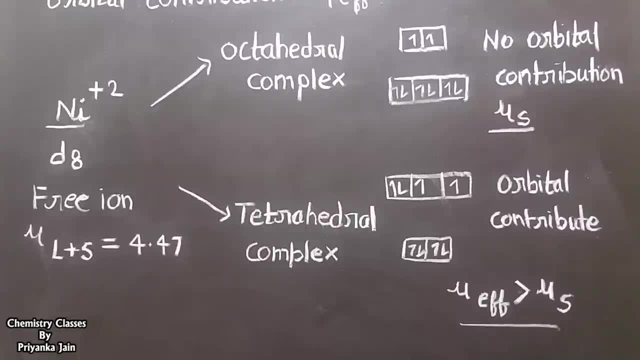 of the complex. Which type of geometry the complex is? taken, For example, if we see the nickel plus 2 ion that has d8 configuration in the free ion state it has both L and S coupling. It means its magnetic movement is given by the combination of both the orbital. end and the free end. So it is given by the combination of both the orbital end and the orbital end. So it is given by the combination of both the orbital end and the free end. So it is given by the combination of both the orbital end and the free end. So it is given. 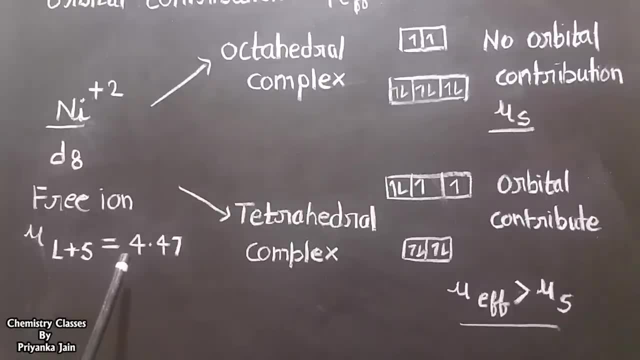 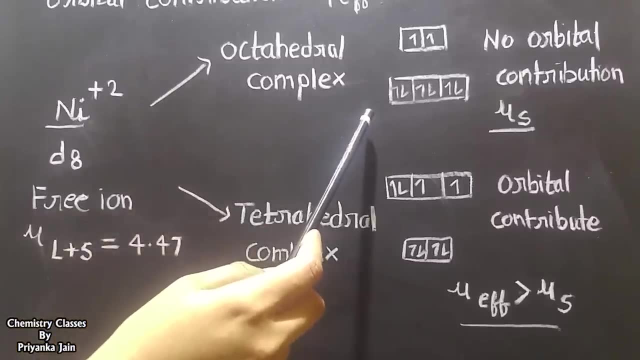 by the combination of both the orbital end and the free end. So it is given by the and the spin contribution and it will be equal to 4.47.. But it then makes the octahedral complex. This is the splitting in the octahedral complex and these T2G levels all are filled. 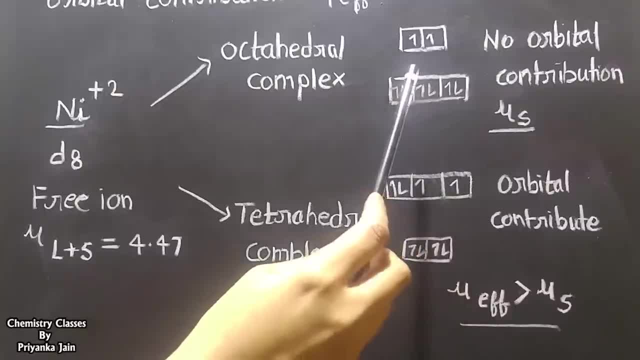 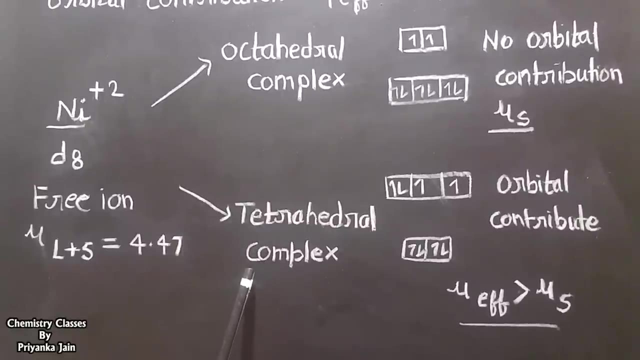 completely. So there is no path for rotation and this complex do not make any orbital contribution toward magnetic movement, So its magnetic movement is given by spin only formula. Now, when it makes the tetrahedral complex, As you know, in tetrahedral complex the splitting is: 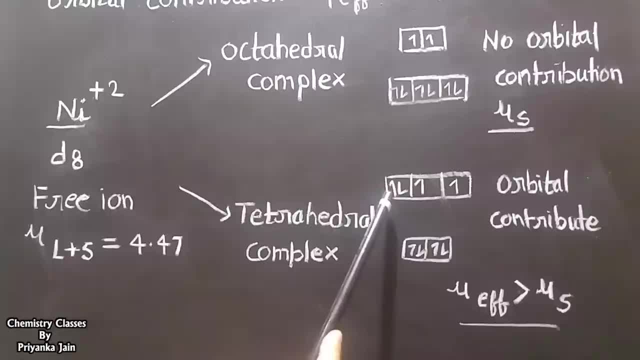 inverted. It means EG label is downward while the T2G label is upward. This is highly in energy. So this type of configuration is found in the tetrahedral complex and this is the T2G label. You can see there is two electrons in this orbital, while one one in these two orbitals. 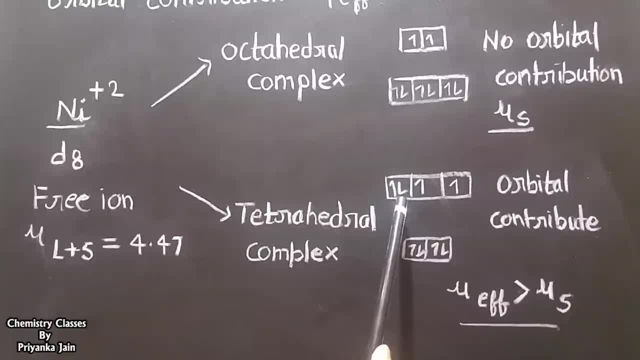 So this electron with the inverted spin can find a path to rotation via this orbital or this orbital, So it can rotate and it makes a contribution towards the magnetic movement. So there the mu effective will be greater than the mu s. It is higher, So by this we can easily 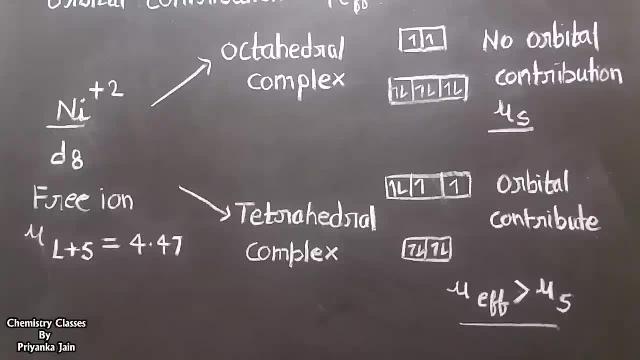 see that which will be the magnetic movement, How much magnetic movement A compound will have when it is complexed or it is not complexed. So you can easily determine by this. Thank you for watching this video. If you like this video, please share. please subscribe. If you want any more topic, you can send us.